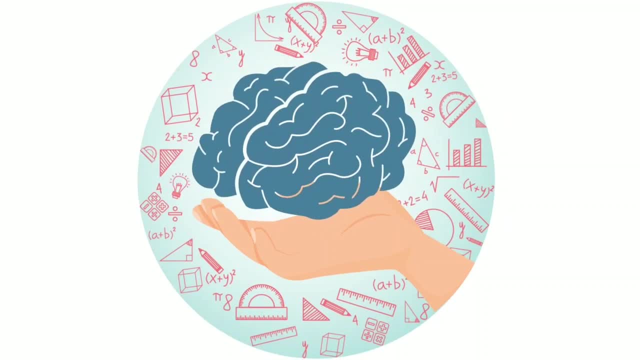 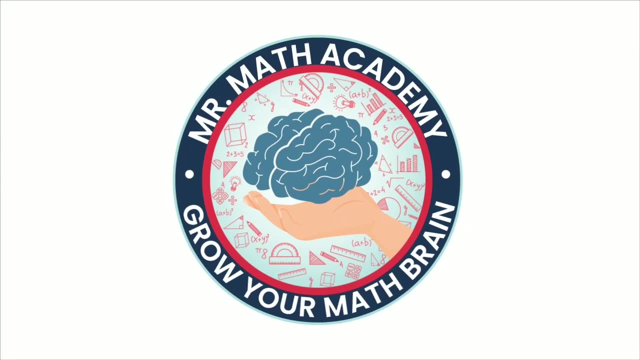 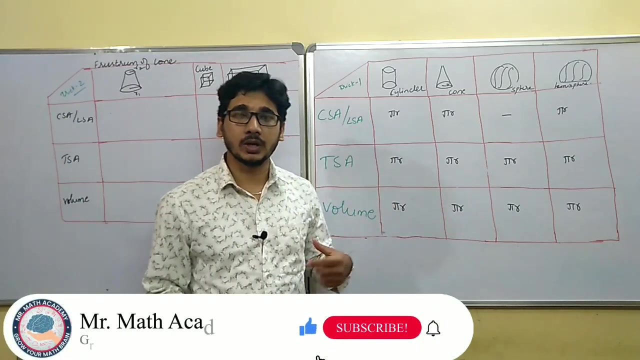 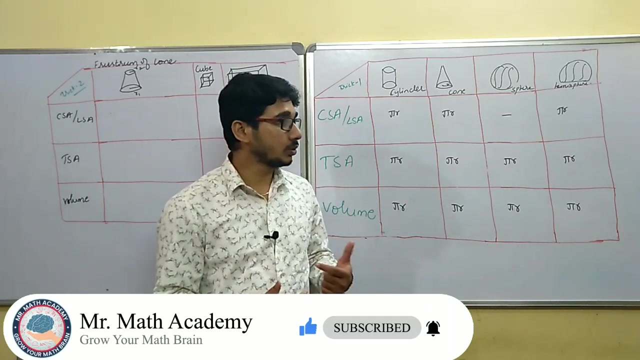 welcome to mr math academy. grow your math brain. welcome back to mr math academy, media students, and let us go for to write the formulas of surface area and volume. okay, in the sense, so already i told you one poem, so what is that? let me write that poem so that, if you remember, 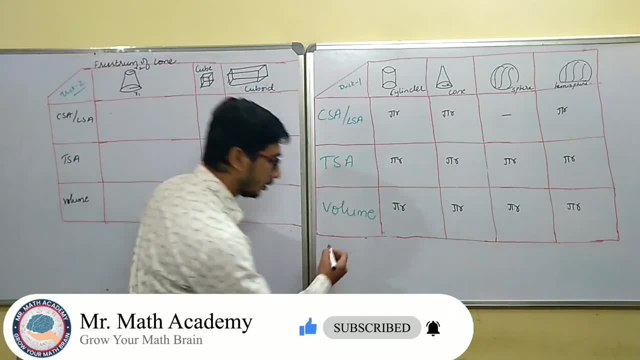 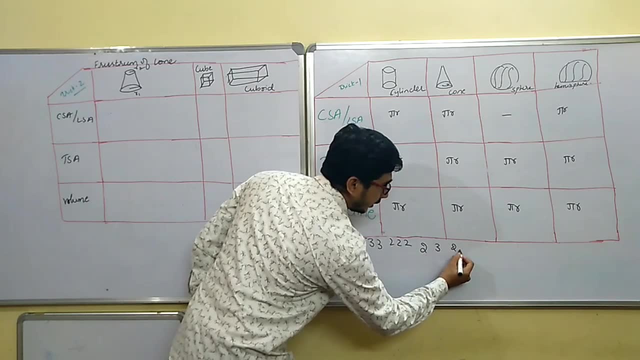 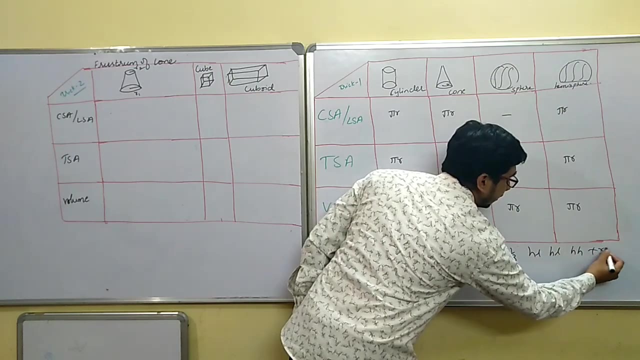 that poem. we can write all the formulas quickly. so what is the poem? so two, two square square cube, cube square square square two, three, two by three, four, four by three, one by three, h, l, h, l, h, h plus r plus r. this is the poem you have to remember. if you remember this poem, you can write. 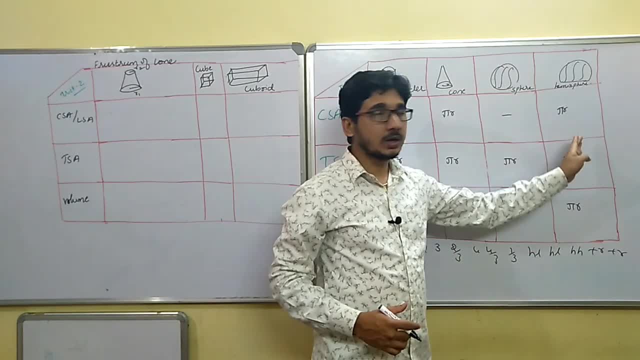 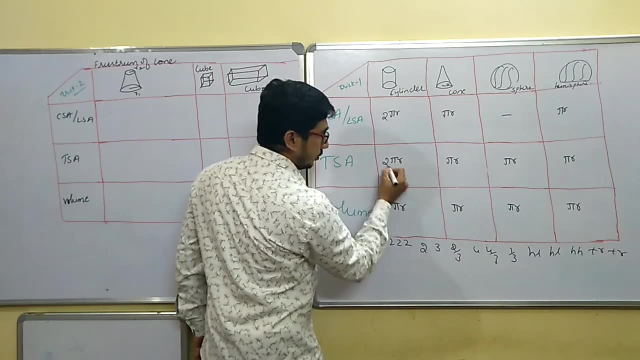 all the formulas quickly. how just you have to go like this: come back: one, two, three. one, two, three, five, seven, eight. you have to remember all this пример of the final danny executives, Probleme and Konadasdir: two, two, square, square, cube, cube, square, square, square, two, three. 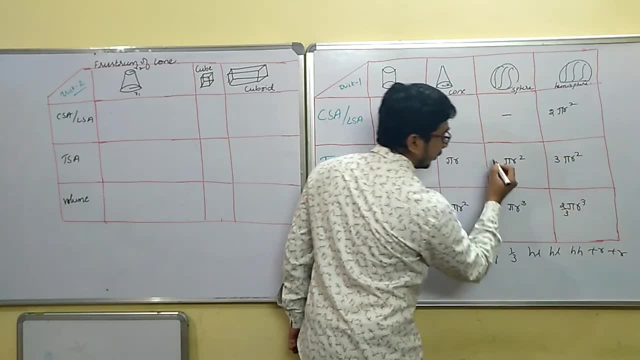 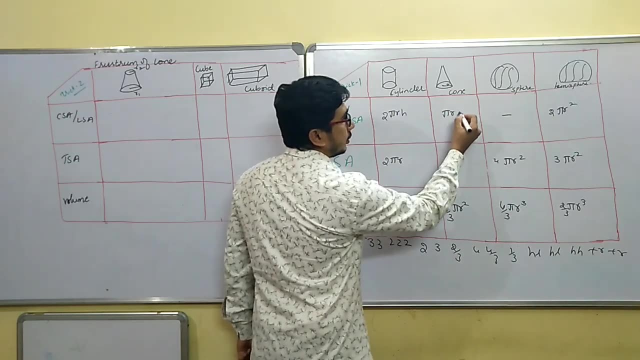 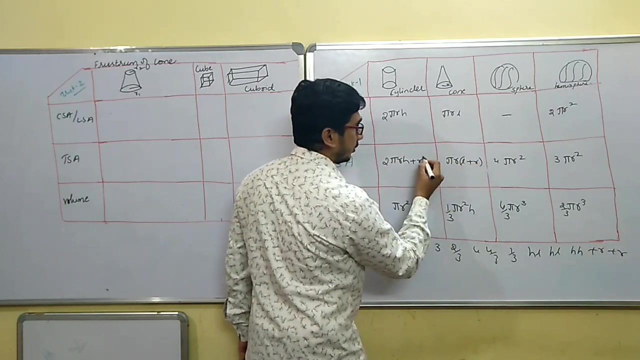 three, two by three, four, four by three, one by three, three, three, three, remember okay, h, l, h, l, h, h plus r, plus r and a bracket. that is all okay. i repeat again: two, two, square, five, square, cube, cube, square, square, square two, three, two by three, four, four by three. 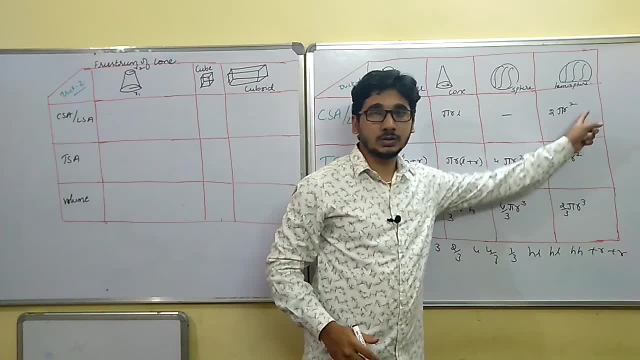 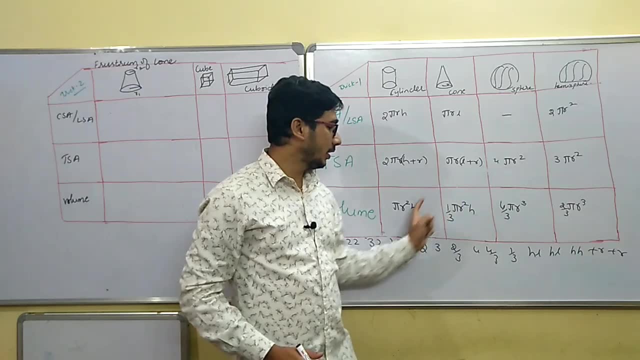 square square cube, cube square square square 2, 3, 2 by 3, 4, 4 by 3, 1 by 3, h, l, h, l h h. 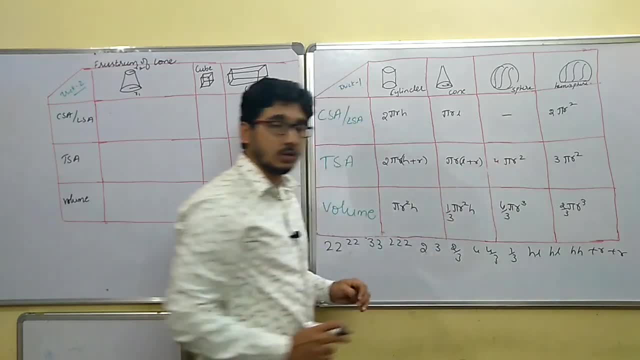 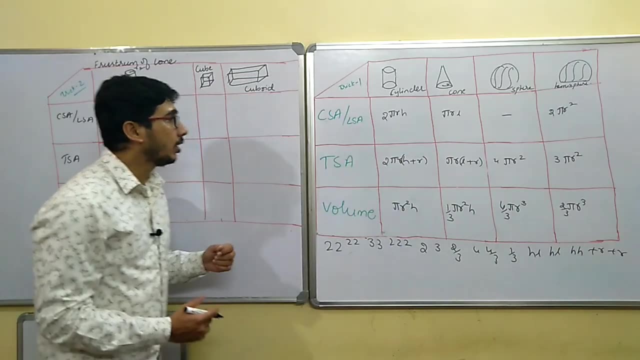 plus r plus r under bracket, finish all the 11 formulas. okay, so you have to remember this poem. so from cone only we will generate frustrum of cone. how see r1 and r2, two radius are there. 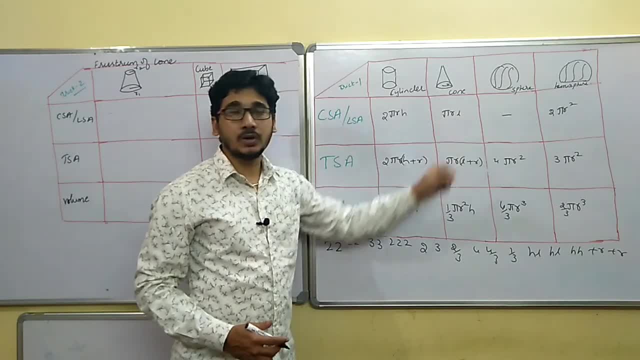 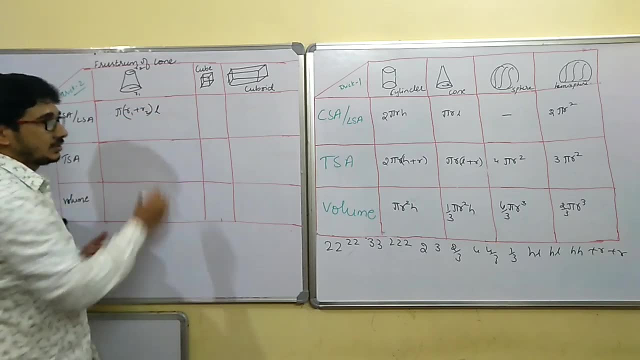 same thing. you copy: pi. r is pi. rl is in the place of r. write down r1 plus r2, so pi r1 plus r2,. under bracket you write down l as it is so. same thing in the place of r. write down r1 plus. 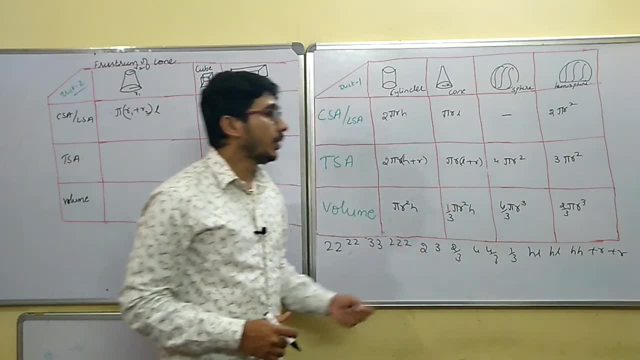 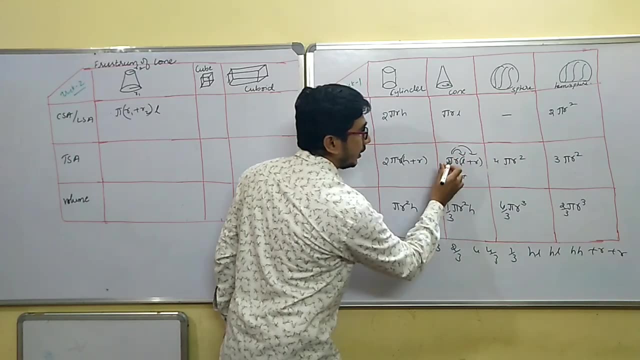 r2, over my dear students, let us go for this one pi r into l plus r. first, I will multiply this pi? rl. if you multiply pi r into l pi rl, pi r into r pi r square, okay. 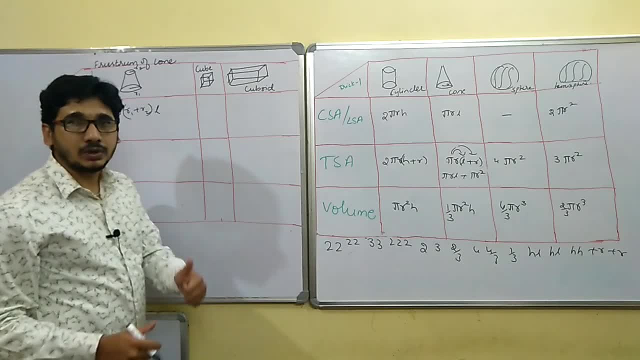 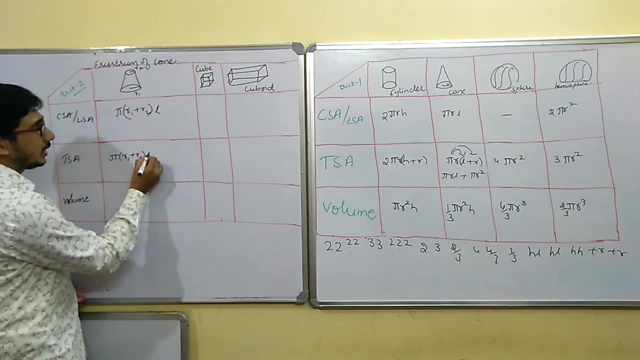 so let me write here in the place of r, write down r1 and r1 plus r2, that's all. so what it will become? pi r1 plus r2, l as it is plus this one pi r square is there. 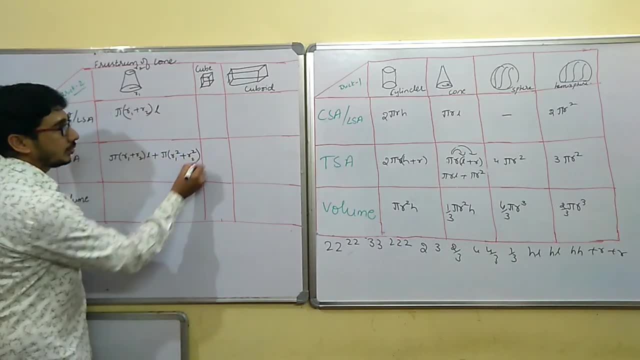 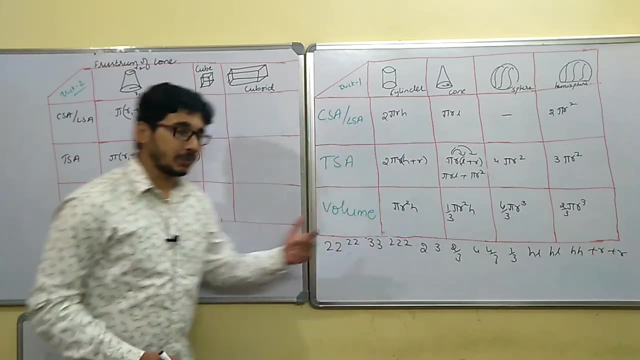 pi r1 square plus r2 square. finish. let us go for volume. what is there? 1 by 3 pi r square h. no, 1 by 3 pi h, write separately. 1 by 3 pi h, write separately. 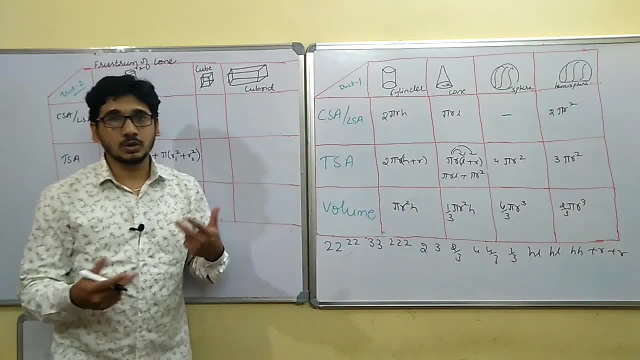 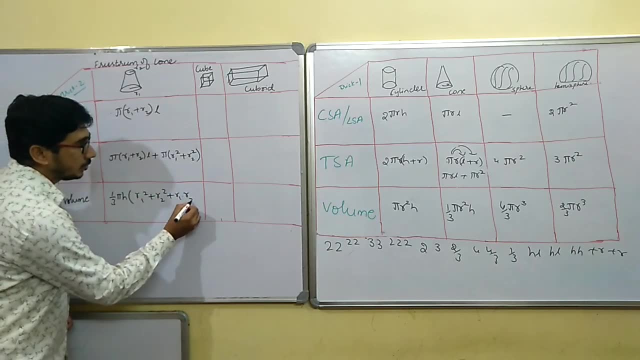 what is there? 1 by 3 pi h- write separately. 1 by 3 pi h- write separately. what is there? r is there? no, in the place of r square, r1 square plus r2 square, one small point we have to remember: r1 square plus r2 square plus r1 into r2,. 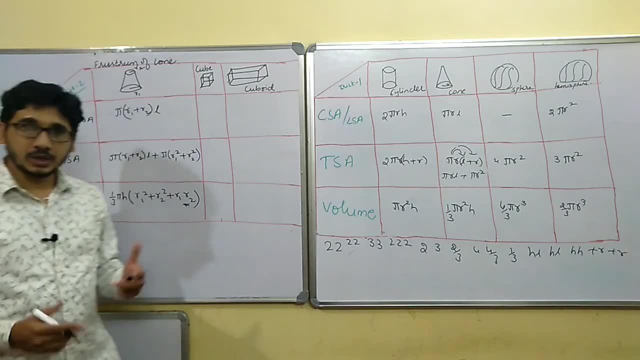 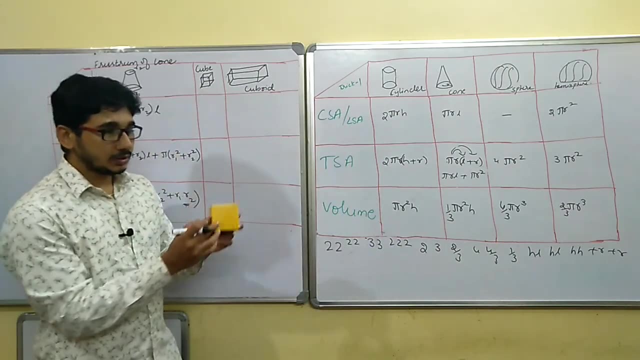 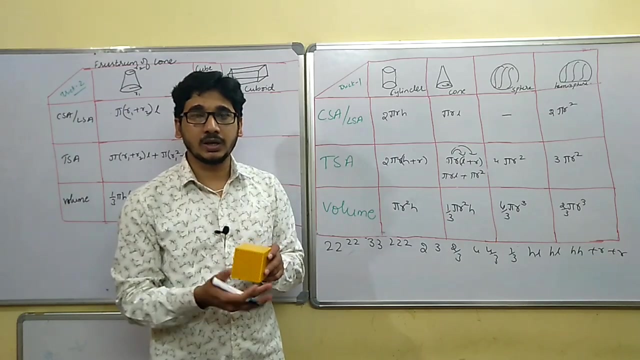 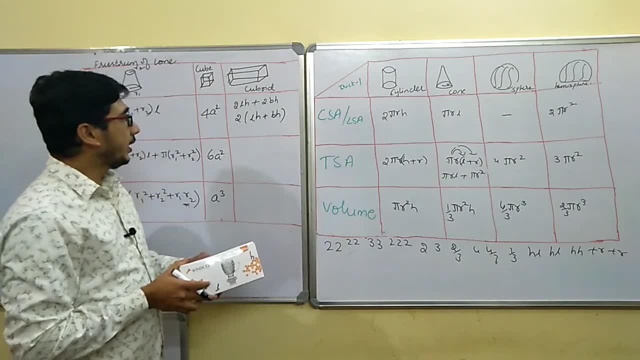 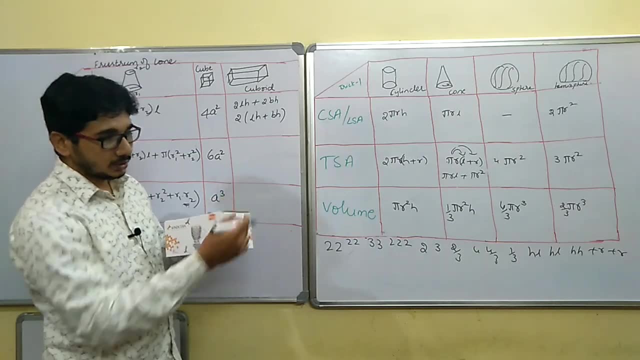 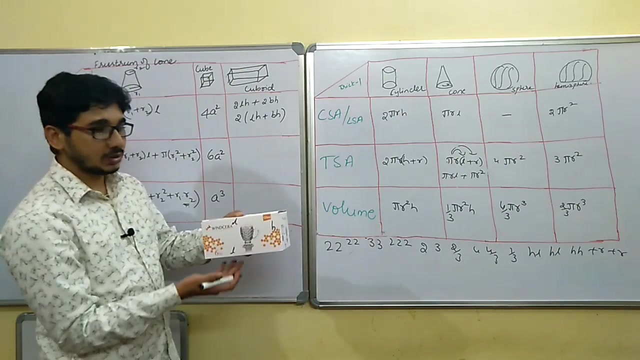